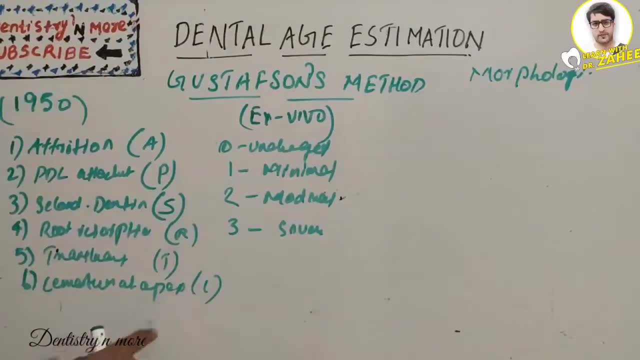 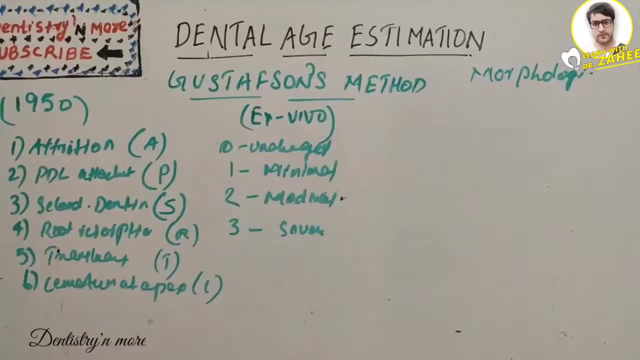 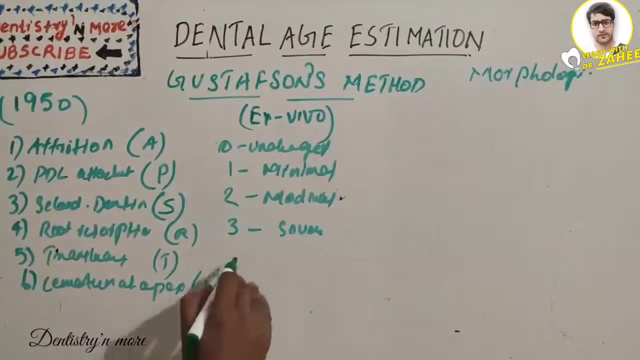 if it is moderately at treated, we are going to put score two. if the root reservoir option is moderate, we are going to put two. if the cementum at apex is more four, we are going to give three. So likewise, we are going to finally get a score. ok, that is. 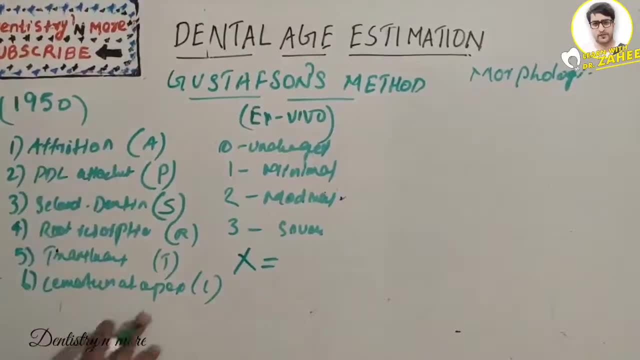 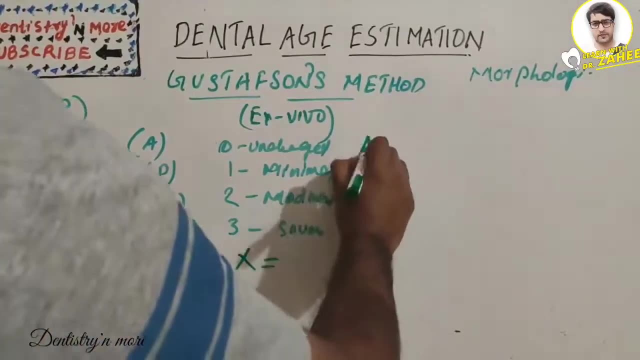 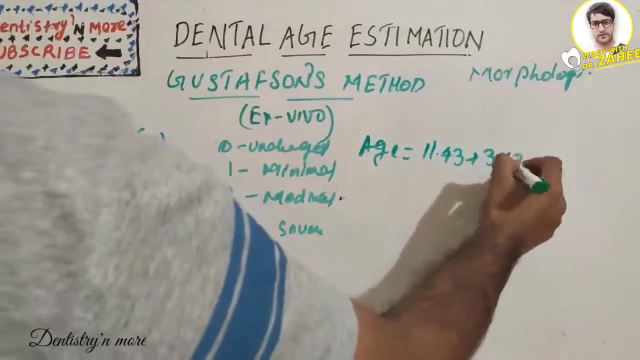 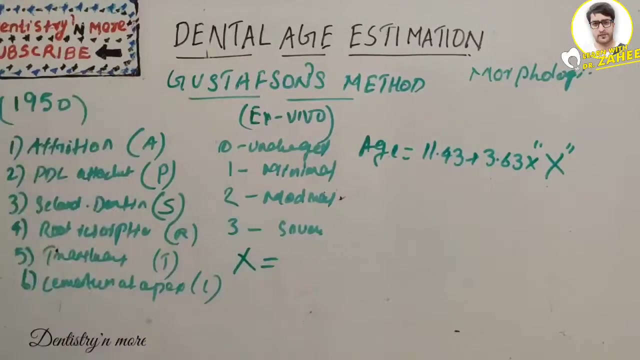 score x, we get a score X, okay. and finally, we get our age by a formula that is 11.43 plus 3.63 into X. so this X is here we get by doing all this calculation, okay. so this is how we calculate Gustafson's. 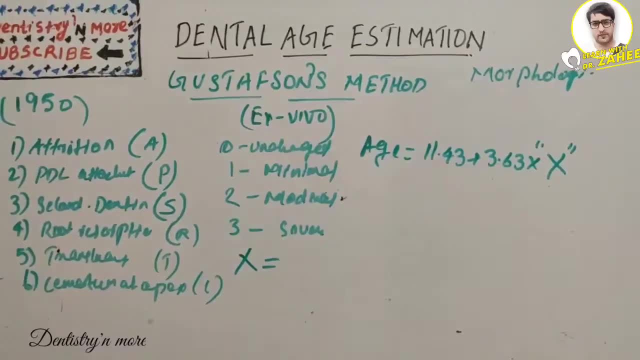 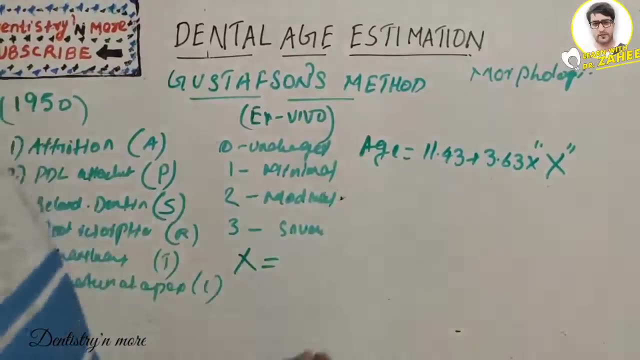 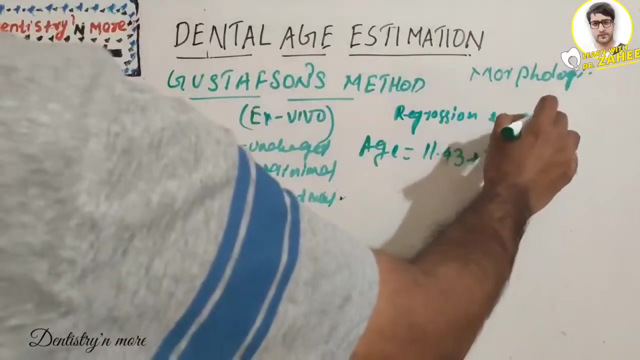 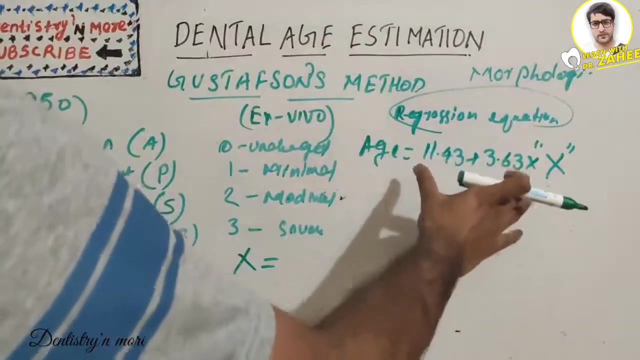 method of age. so you might be wondering where this 11.43 and 3.63 came from. this is actually a regression equation. it is a mathematical regression equation put forward by this Gustafson. okay, so it has finally reached to a standardized value. this is a constant and this 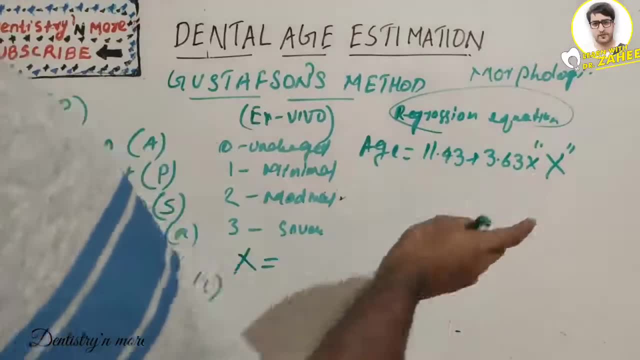 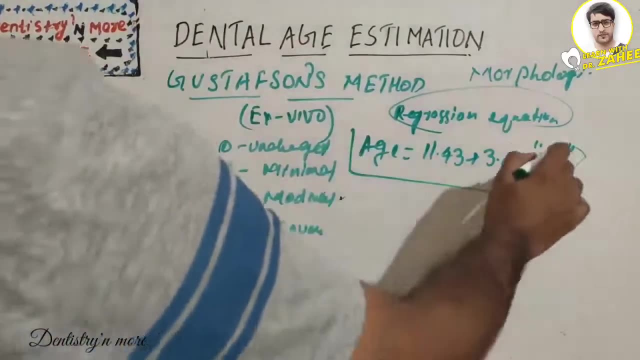 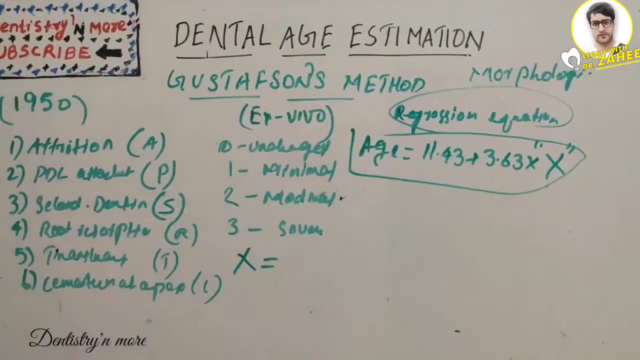 is a coefficient. so you can put any equation in the equation and you can put any equation X value and we will get a generalized population age. so that is how this regression equation works. so Gustafson's regression equation is this one: 11.43 plus 3.63 into the into X, whereas 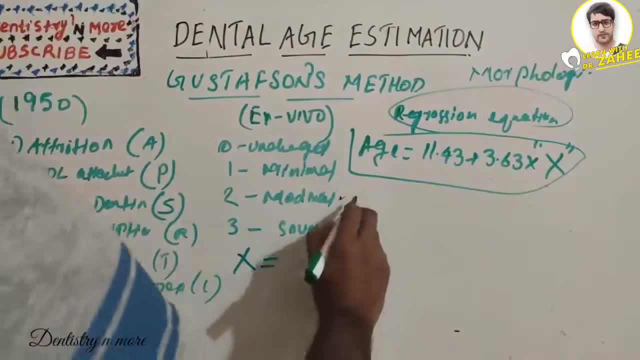 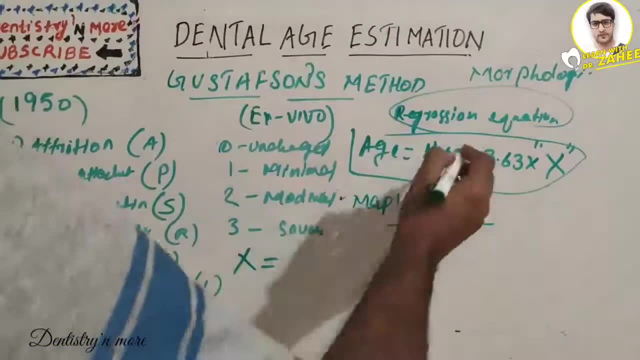 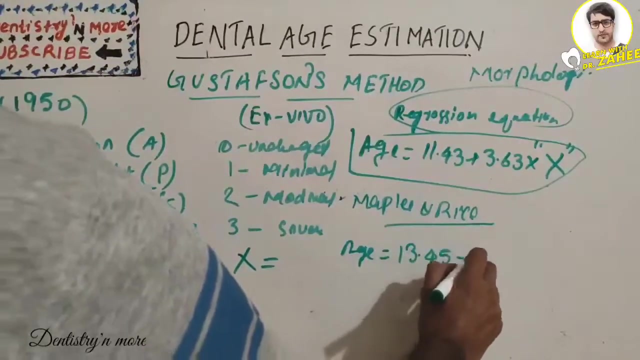 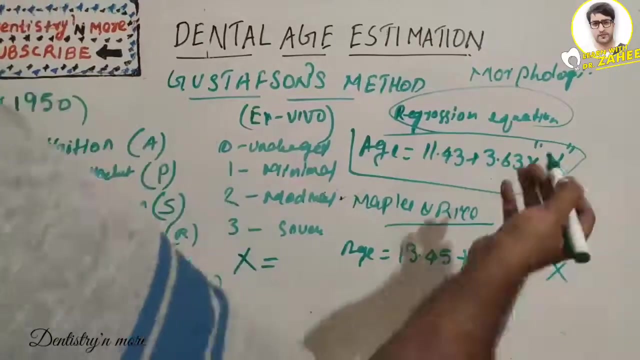 the maples and rice corrected this formula. maples and rice, two scientists corrected this formula. they changed. the constant value, that is age, is equal to 13.45 plus 4.26 into our X. so suppose this X is 5, we are going to multiply 3.63 into 5 and 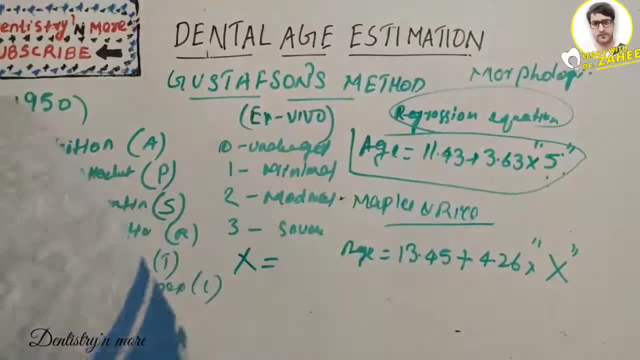 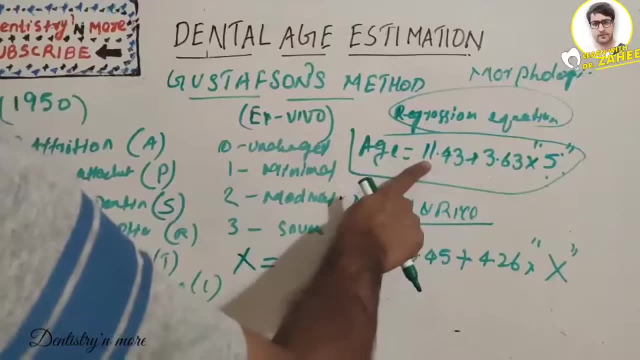 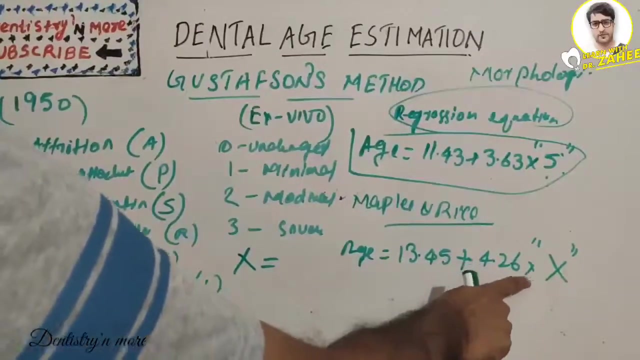 add to this 11.43. okay, so in this case it will be increased. here both the values are more in place. he said it is, or it should be, 13.45 and 4.26 into this 5, so we get any number of X in a particular. 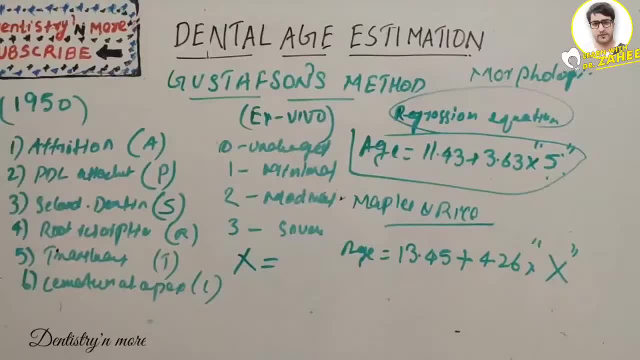 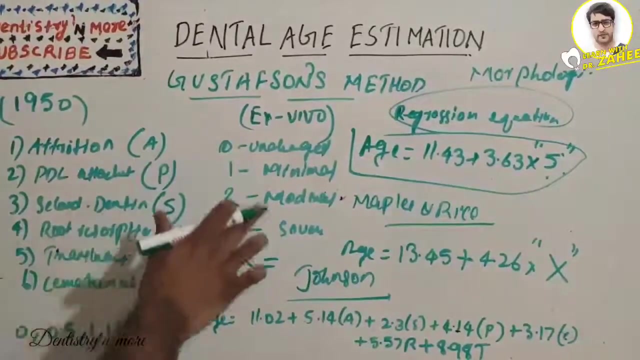 it changes from person to person, whereas Johnson Johnson has again modified this formula. Johnson modified the formula like this before that he modified the scoring numbers, that is, 0, 1, 2, 3, modified into 0, 0.511.52.5 and 3. he added a point five in between and he completely. 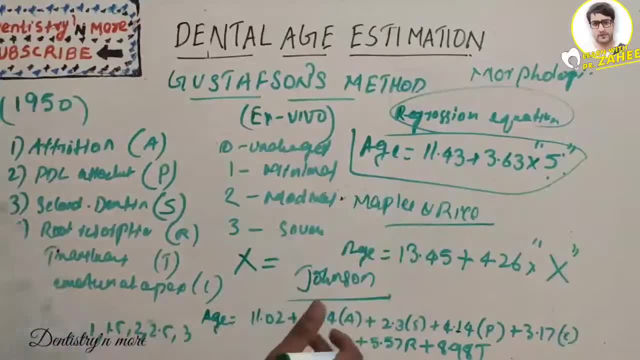 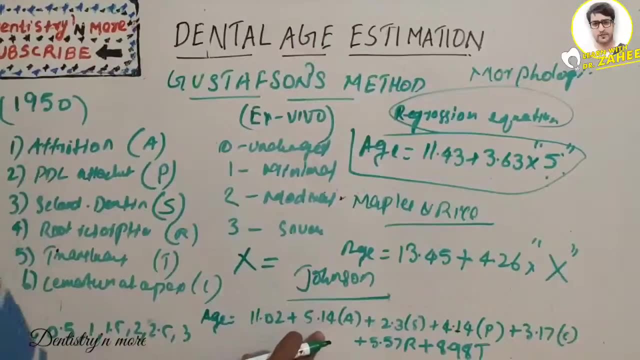 renovated this formula. as 11.02 is a constant, then each value will be added with a coefficient that is 5.14 into the value of a, 2.3 into the value of S, 4.14 into the value of t to the value of s 244.47.. we are adding the value of a 2.3 into the value of s 64.17.. 5.14 F is negative, so now what we have to do? we have to multiply it, so as we have multiplied the value of a 4.3 into the value of s 24.17.. 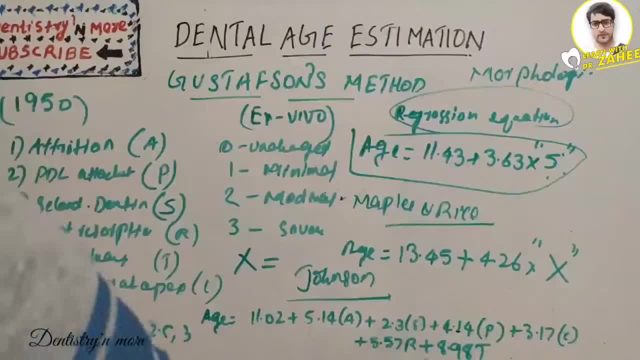 by adding the value of s 4.14 into the value of s 4.17.. then 3.17 to the value of c, 5.57 into value of r and 8.98 into the value of t. so finally we get. 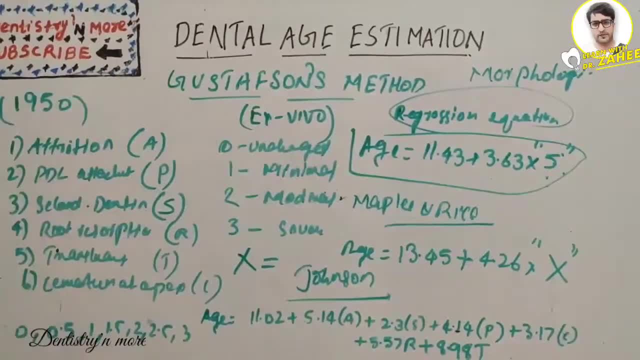 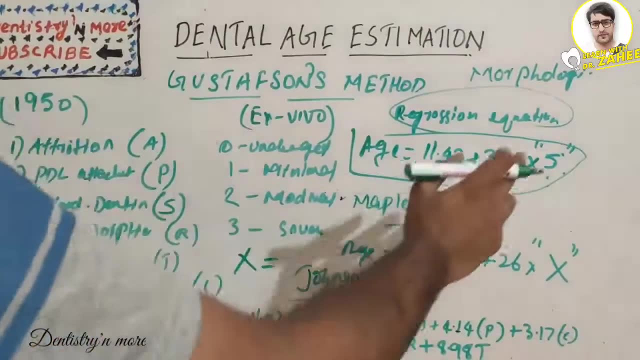 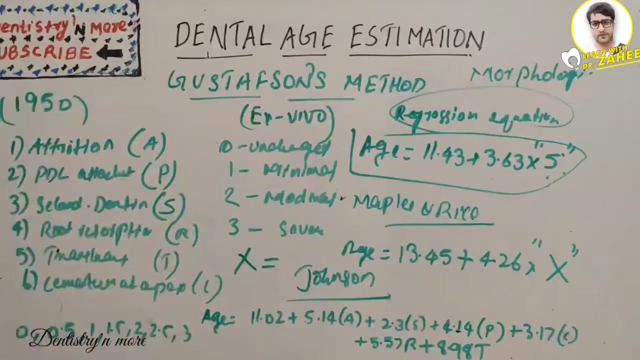 the h. so this is a mathematical regression equation: first gustafsson modified, 11.43 plus 3.63 into x, then maples and rice, 13.45 plus 4.26 into x, but johnson completely renovated, that is 9.0 into all this each will be separately multiplying with the regressive changes. so this: 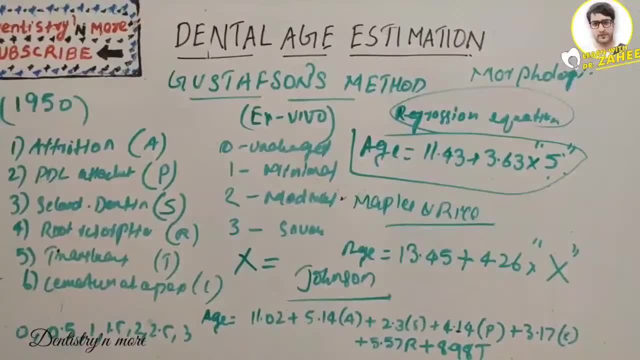 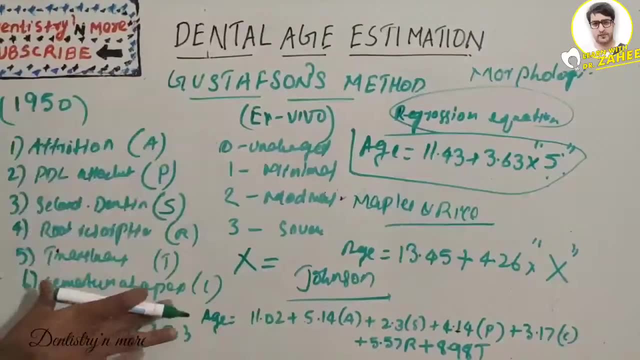 is how we calculate gustafsson method. so this method is basically directly: we do examination, morphological examination, on the six criteria with a score of 0, 1, 2, 3, and we get the score of x and we apply it on the equation or johnson's method, whereas 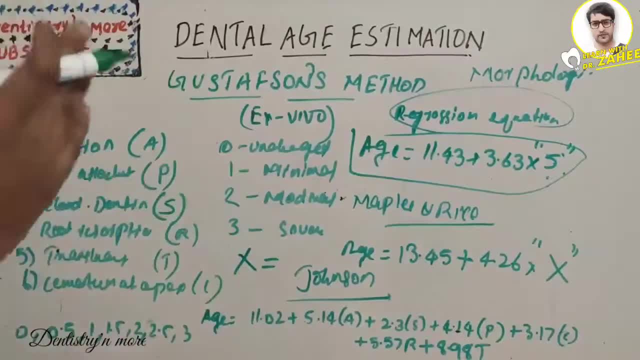 the, the, the. the first one. what we studied is the demigian's method. it is a radiographical method. we calculated by various stages and converting into score and adding up the scores and comparing with the standardized table. so that's all about two methods: gustafsson and demigian's method.